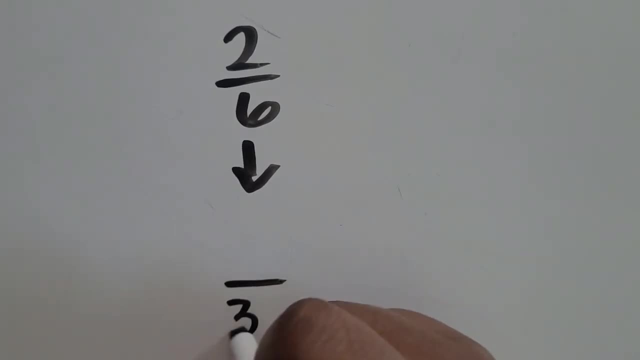 Last, let's work on 2 sixths. How many groups of 6 equals 30? 5. 5 groups of 6 equals 30 or 5 times 6 equals 20. Let's do the same for the numerator. 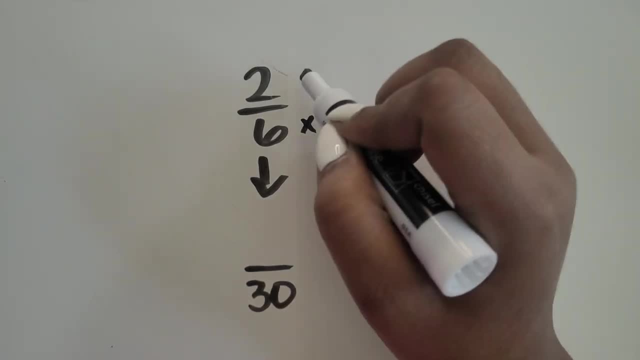 5 groups of 2 equals 7 or 7 equals 8. 5 groups of 2 equals 12 or 5 times 12. Remember ourcla? Let's put everything together then stop here and add a number to find all of 1 as equal. 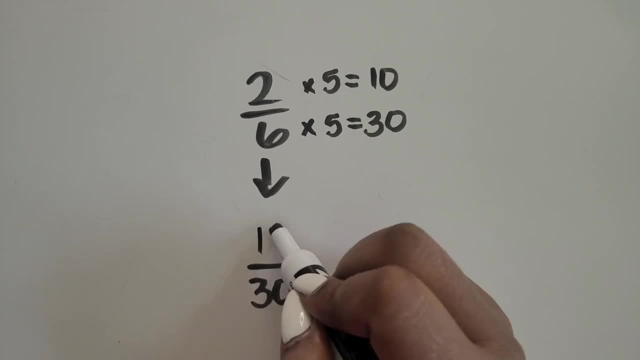 For each number, all the enemy items are almost always sums. So, we'll just use a number immediately, to nice you'll weMaddy go. Number two, 5 groups of 7 equals 10 equals 10 is this. If None equals 10, or 5 times 2 equals 10. Now that we have equivalent fractions to the original fractions 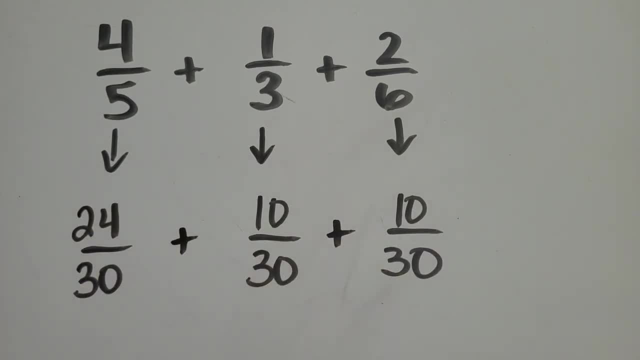 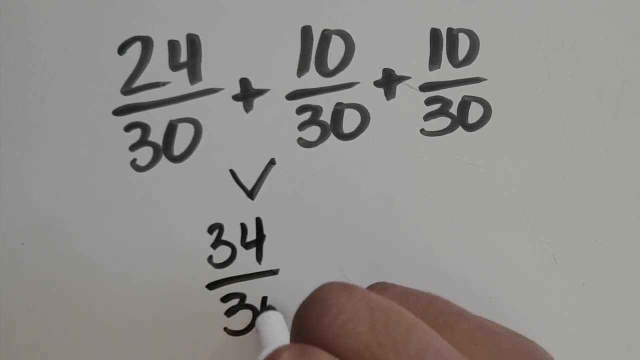 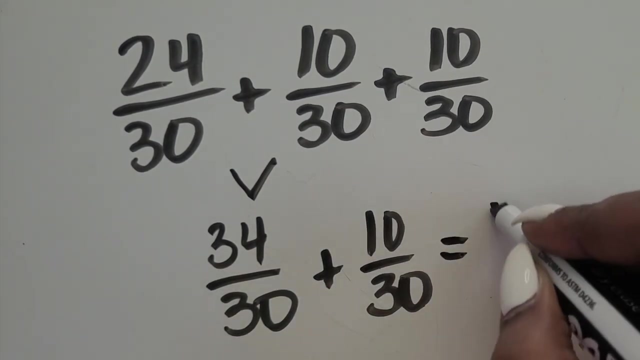 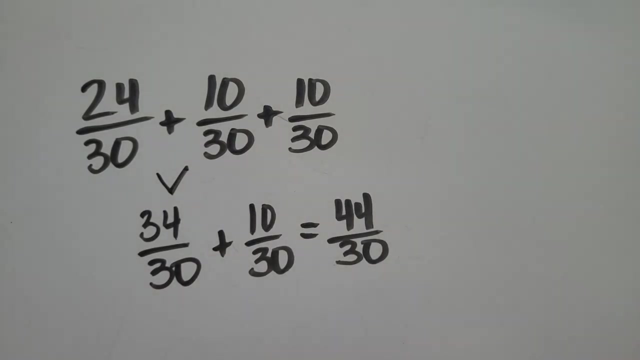 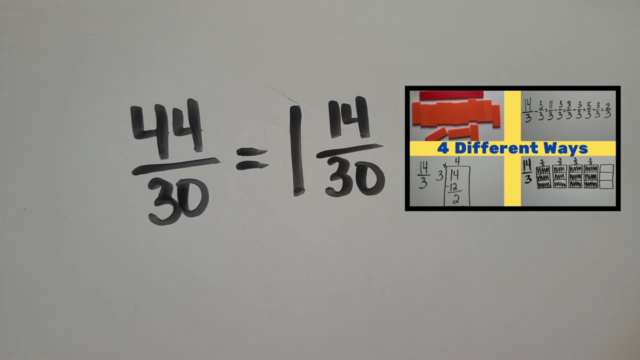 with all common denominators, can we add them together? Yes. 24 30ths plus 10 30ths equals 34 30ths. 34 30ths plus 10 30ths equals 44 30ths. The sum of the fractions is 44 30ths. We can rename this fraction greater than 1 as a mixed number. To learn the steps to do this, watch my video on converting fractions to mixed numbers. 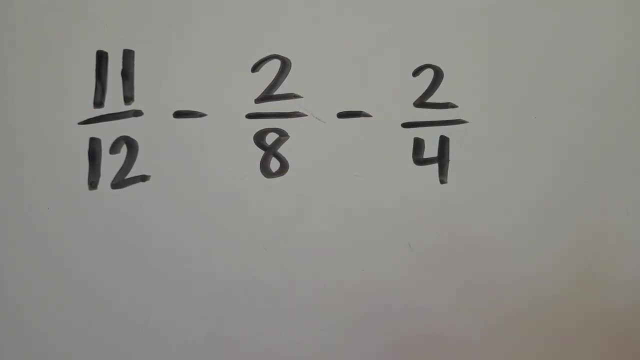 How could your students go about solving a subtraction expression with three fractions? 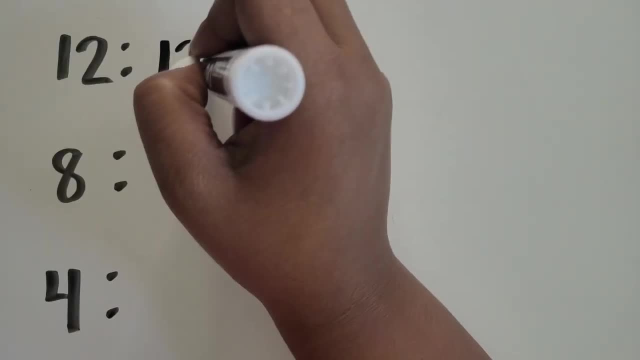 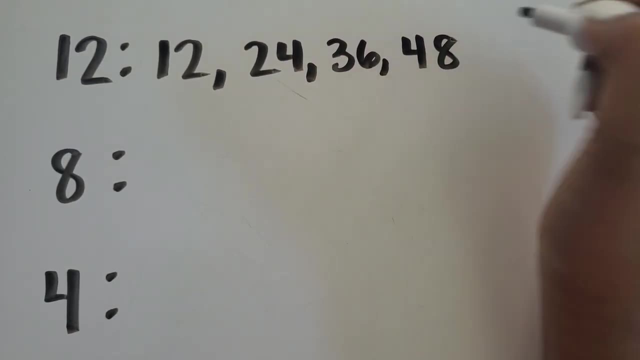 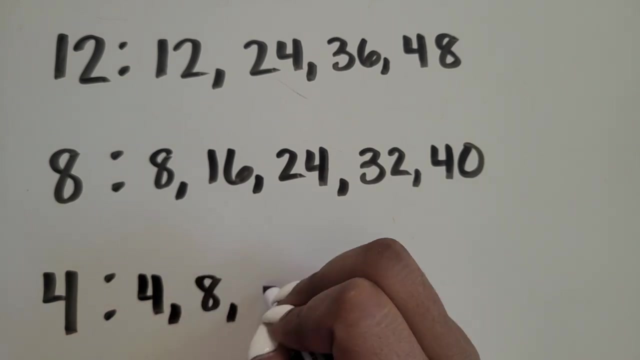 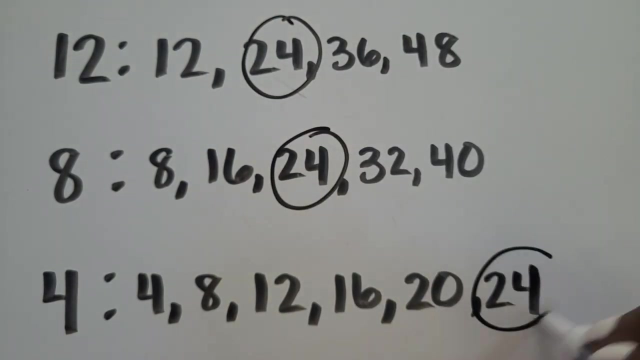 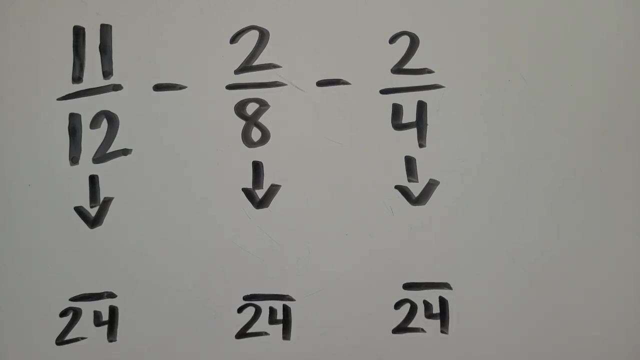 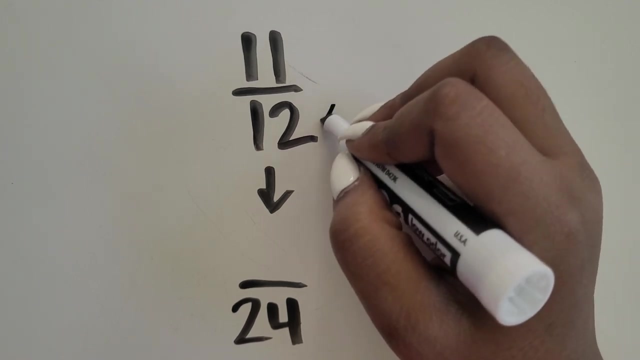 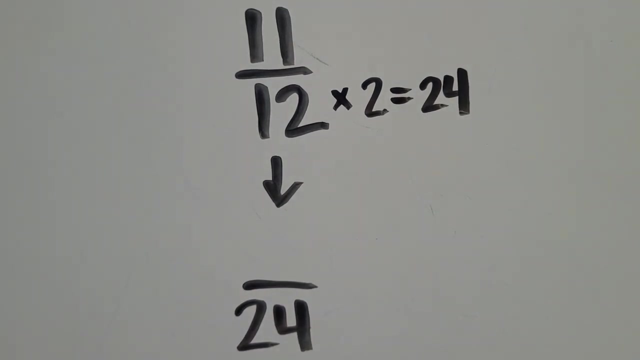 Again, let's list out the multiples of the denominators in order to find a common denominator. For 12, we can list out 12, 24, 36, 48, 8. 16, 24, 32, 40, 4. 4, 8, 12, 16, 20, 24. We can see that they all have 24 as a multiple. So we'll use 24 as the common denominator. Let's find out what each new numerator will be. We'll start with 11 12ths. How many groups of 12 equals 24? 2. 2 times 12 equals 24. Let's do the same for the numerator. 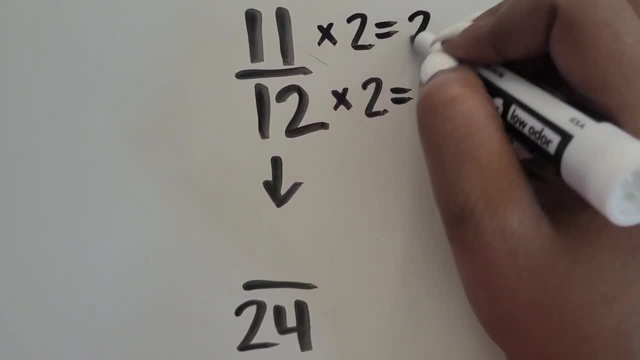 2 times 11, or 2 groups of 11, equals 22. Our equivalent fraction to 11 twelfths is 22 twenty-fourths. 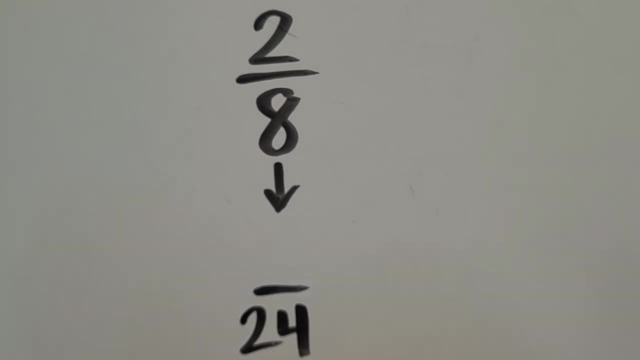 Now let's work on two eighths. How many groups of 8 equals 24? 3. 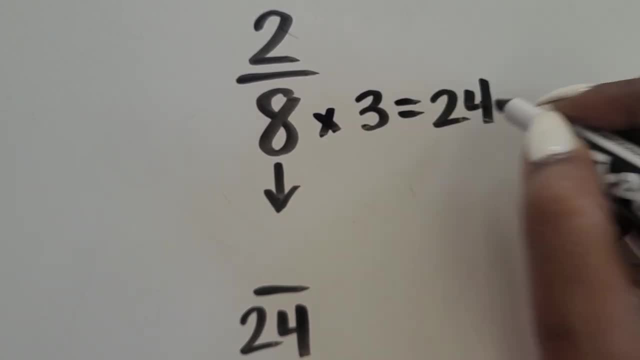 3 times 8 equals 24. 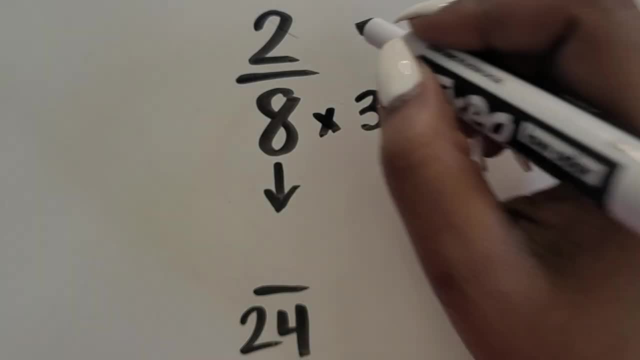 Let's do the same for the numerator. 3 times 2, or 3 groups of 2, equals 6. 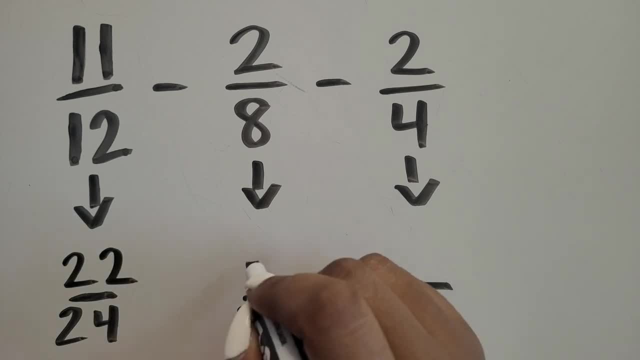 The equivalent fraction for two eighths is 6 twenty-fourths. 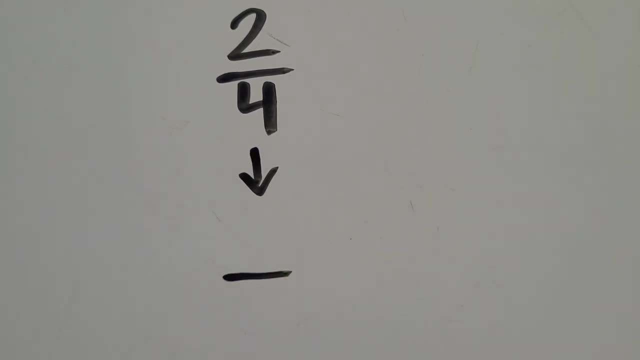 Last, let's work on an equivalent fraction for two-fourths. 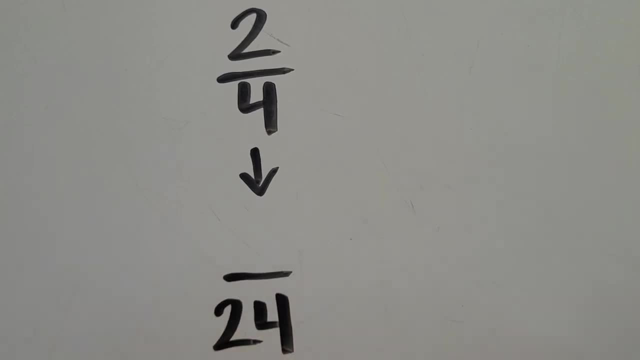 How many groups of 4 equals 24? 6. 6 times 4 equals 24. 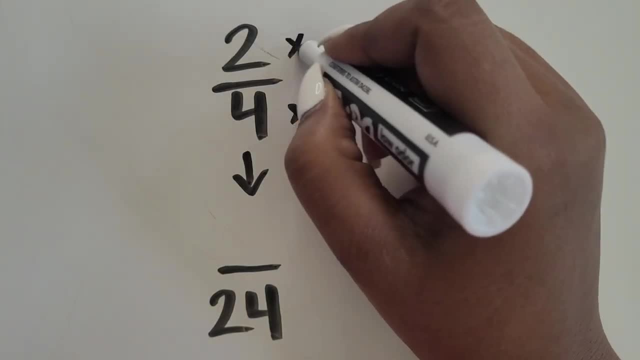 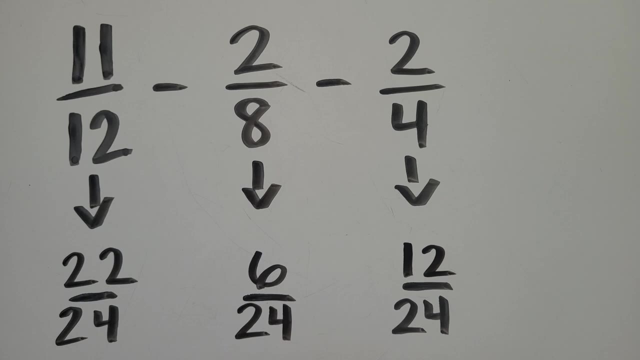 Let's do the same for the numerator. 6 groups of 2, or 6 times 2, equals 12. An equivalent fraction for two-fourths is 12 twenty-fourths. 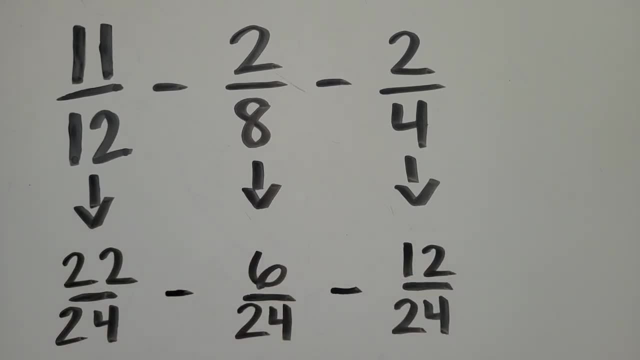 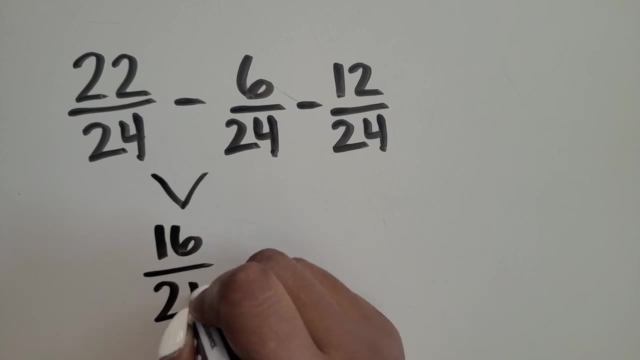 We can subtract now that the denominators are alike or the same. 22 twenty-fourths minus 6 twenty-fourths equals 16 twenty-fourths. 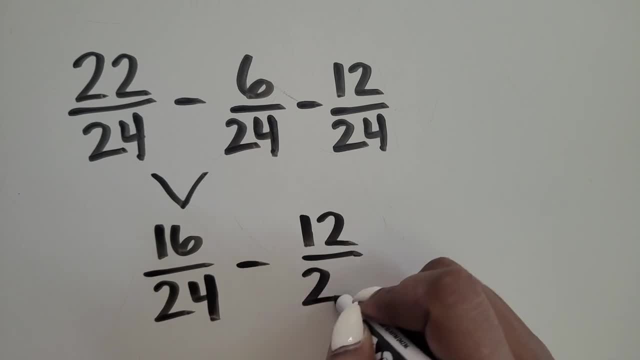 16 twenty-fourths minus 12 twenty-fourths equals 4 twenty-fourths. 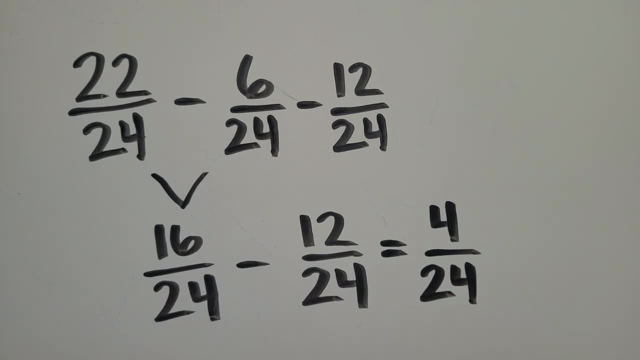 The difference of the fraction. The difference of the fraction is 4 twenty-fourths. 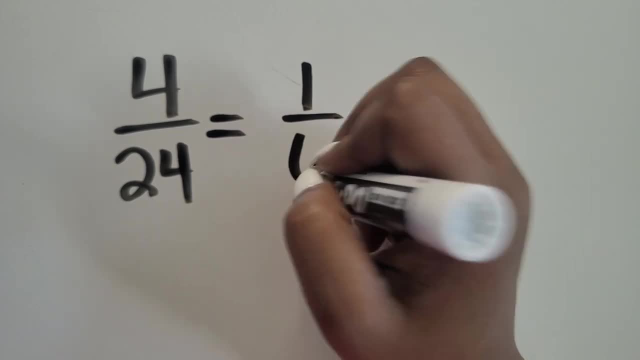 An extra step can be to simplify this fraction. To learn how to do this, watch my video on simplifying fractions. 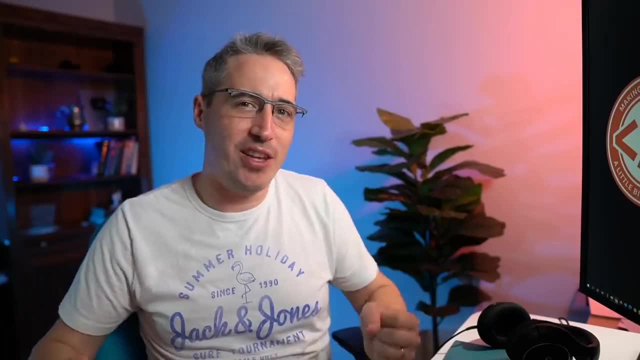 You've done all the hard work to make a really cool layout and then you make your browser window just a little bit smaller and all of a sudden you find something that's overflowing. You let out a bit of a sigh, but then you throw in a media query and you fix that, and then you try changing things. 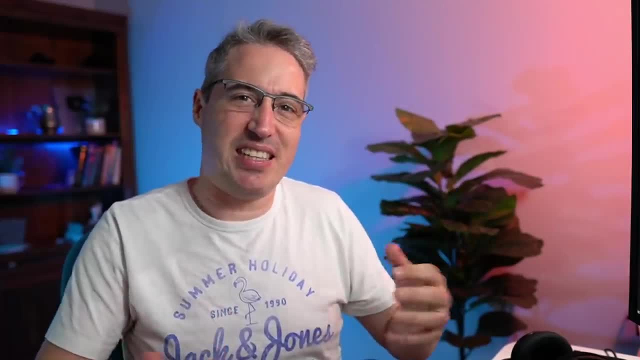 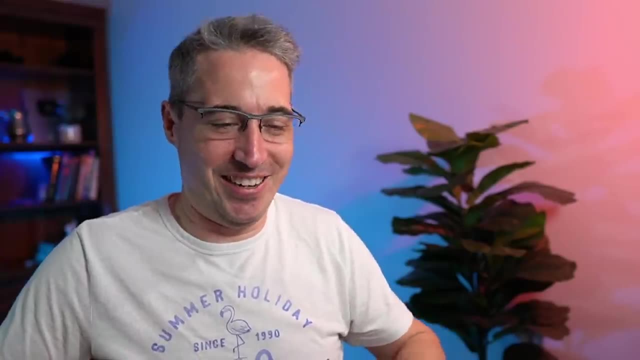 a little bit more. You adjust your browser window a bit just to test things out, and then you find some text that's too big at small screens and you curse to yourself a little bit and you start working on that and eventually you solve that problem. Then you decide to try out what if it's? 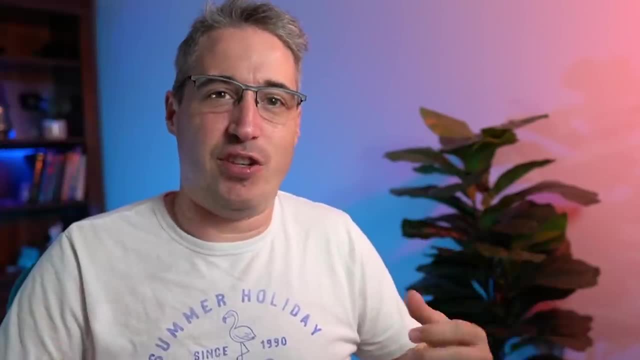 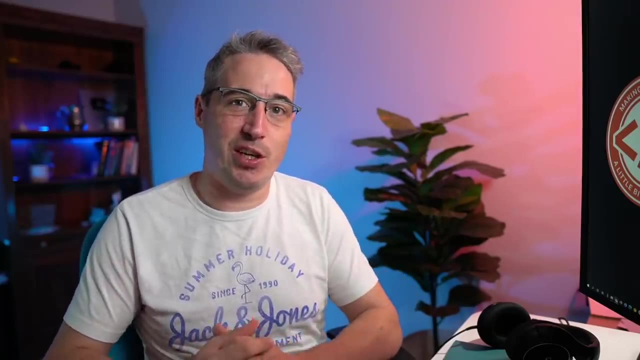 in portrait mode and things just fall apart there as well, and you just feel like throwing your computer out the window. Luckily for us, now we have a lot of modern CSS solutions that do make it just so much easier than it used to be. So in this video, what I'm going to be doing is giving 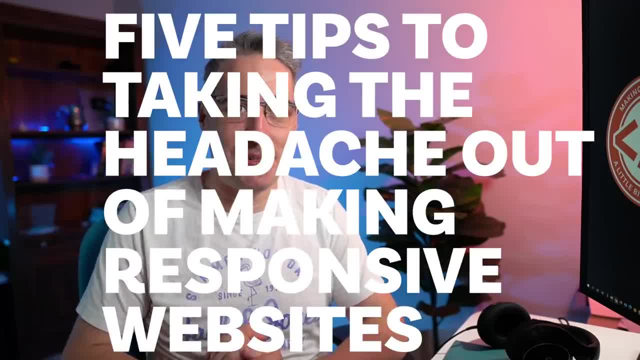 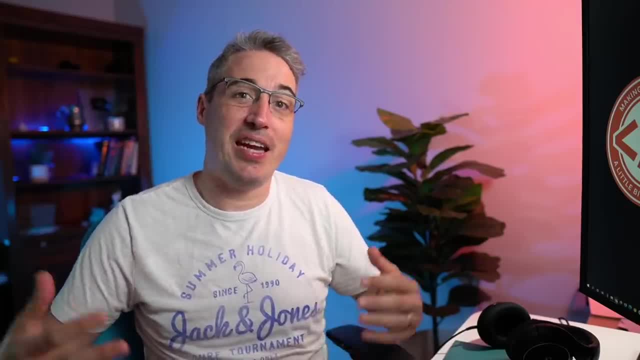 you five tips to taking the headache out of making responsive websites. Hello there, my friend and friends, and welcome back to the channel. I'm so happy to have you here and, if you happen to be new here, my name is Kevin and here at my channel we learn how to embrace the cascade and fall madly.